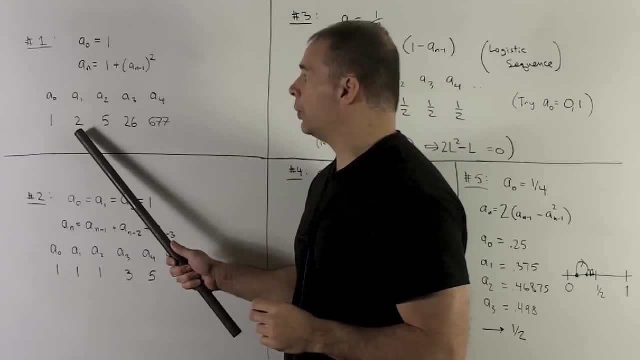 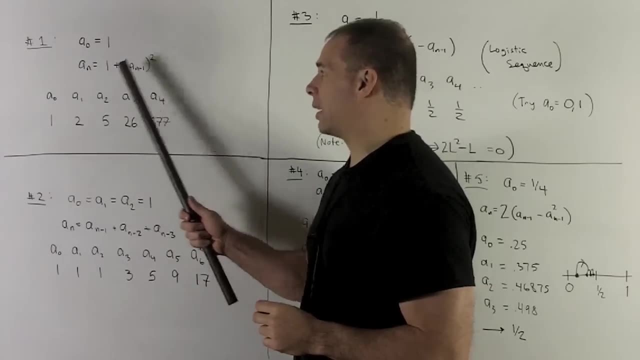 I'm going to take 1, square it and add 1, gives me a 2. Put 2 in there. take 2 and square it, add 1, gives me a 5.. Put 5 in there. 5 squared, add 1, gives me 26,, and so on And 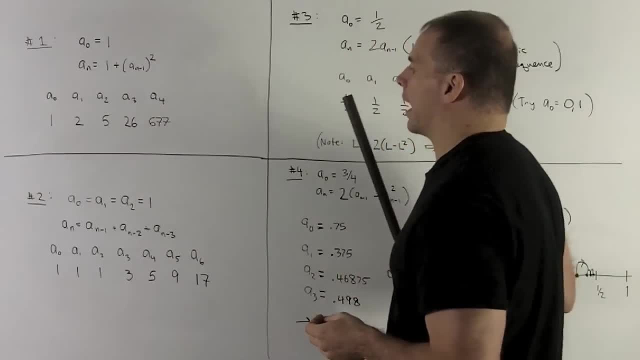 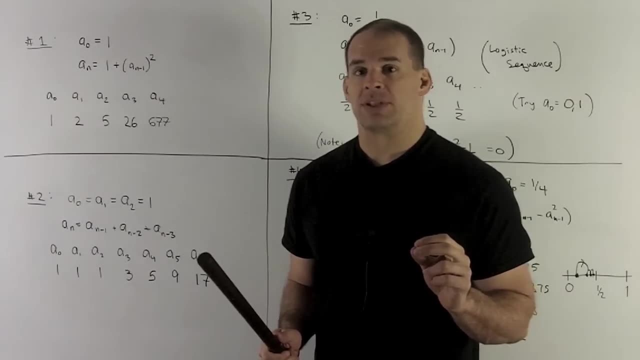 then we note this thing just keeps growing bigger and bigger as we keep moving out. Okay, for another example. so this is a little generalization of the Fibonacci sequence. So here, instead of defining our sequence in terms of the 2 that come before it, 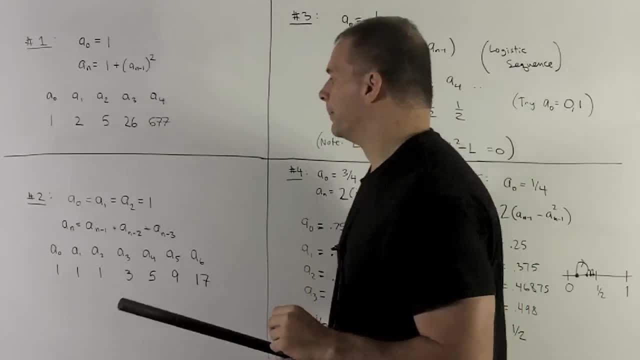 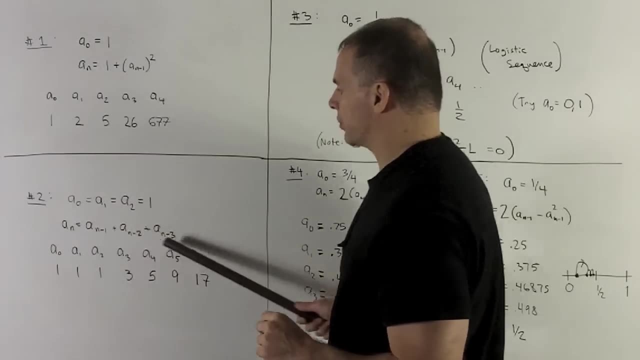 we're defining it in terms of the sum of the 3 that come before it. So a0 equals a1, equals a2 equals 1, and then an is just sum up the previous 3 terms. So we have 1,, 1,, 1 for. 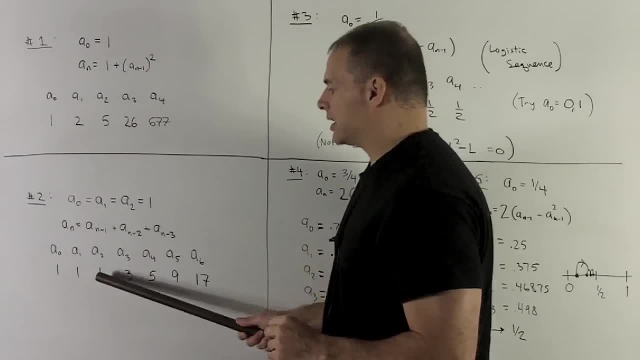 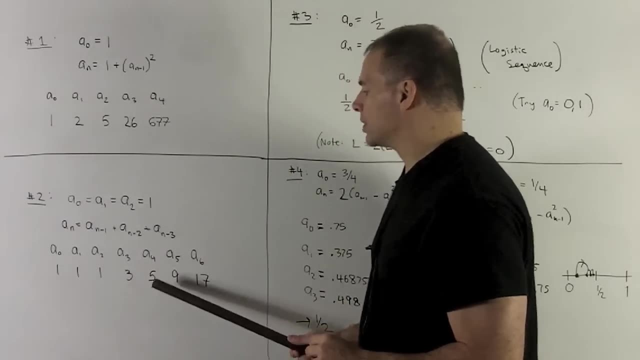 a0 through a2.. Then a3 I get by adding these together, which gives me 1 plus 1 plus 1 is 3.. a4 I get by adding 1 plus 1 plus 3 together, which is 5.. a5 is going to be given by adding. 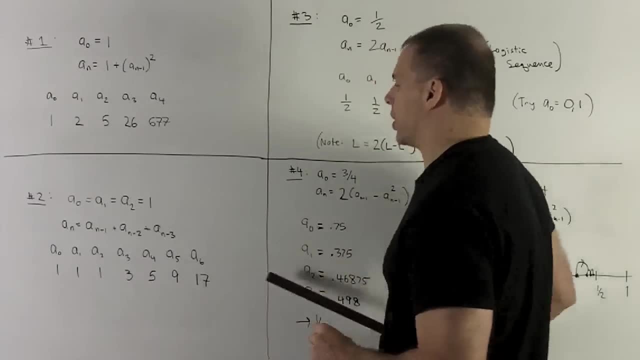 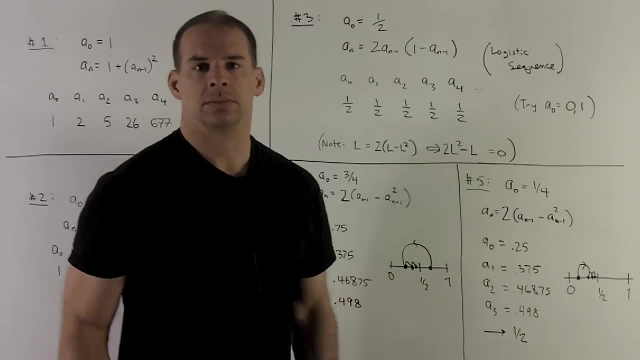 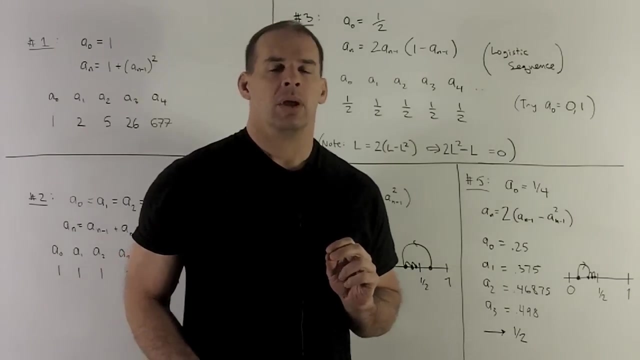 1 plus 3 plus 5.. Which is 9, and so on, And again we'll see that these numbers, as we go out, are just going to grow without bound. So let's look at the problem in a different way. What I want to do here is I want to 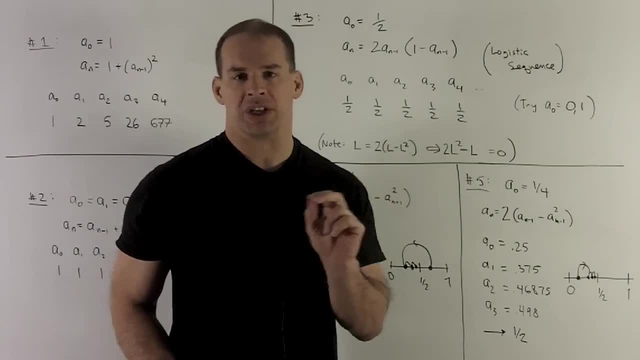 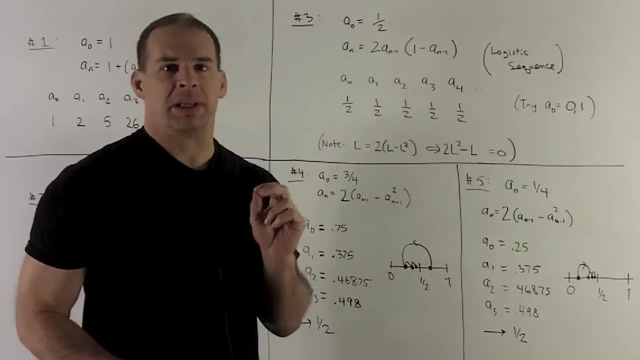 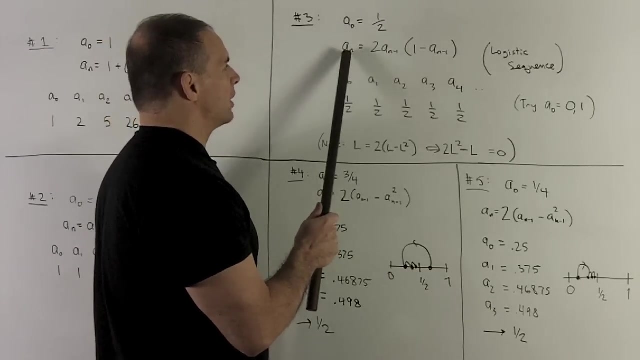 stick with my same recursive relation. I just want to push the initial conditions around. So what I have is what we call the logistic sequence. It's going to come up in population modeling. So our recursive relation is going to be to get my next term in the sequence I take. 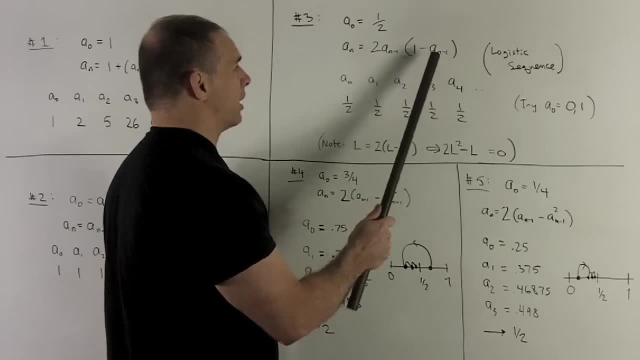 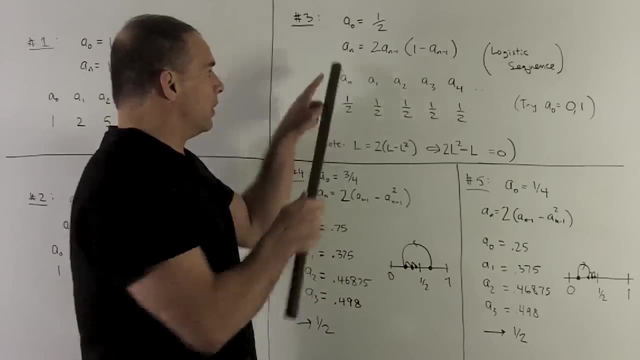 the term before it, then I multiply it by 1 minus the term before it and then multiply by 2 for the example that I'm looking at. Okay, and this will be interesting when the numbers that we're looking at we're starting. 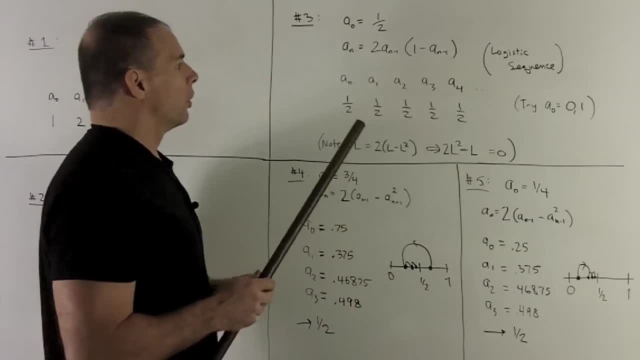 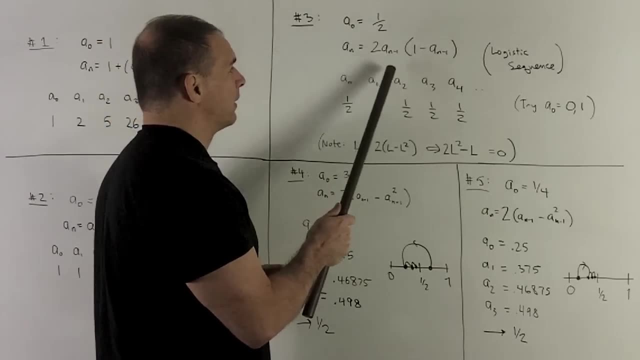 with are between 0 and 1.. Okay, so why don't we start with a half and see what happens? So if I put a half into here, it's going to be 3 times 1 minus a half, so that's going to be 2 times. 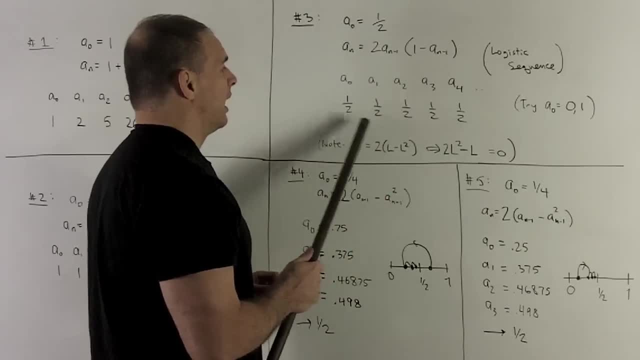 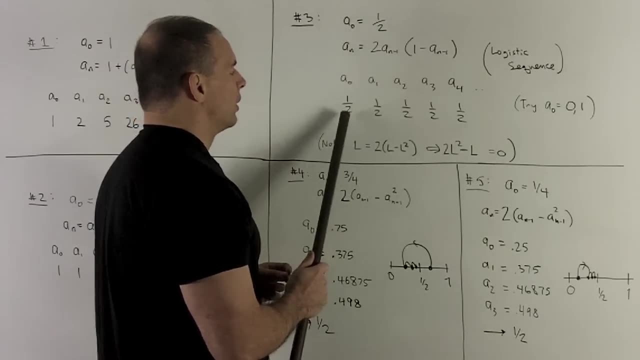 which is 1, times a half. So half goes in, half comes out. Alright, well, we're going to put a half back in. so half goes in, half comes out. And you'll notice if I start with a half. all we can do is keep producing a half until 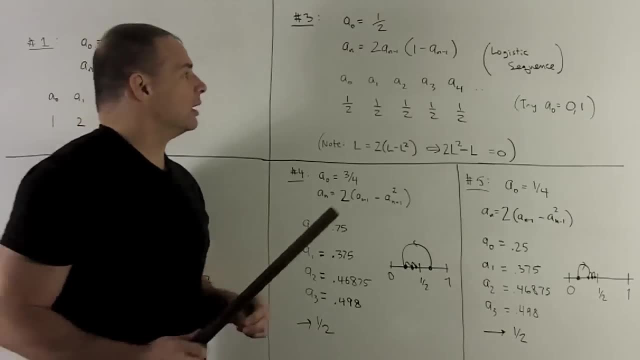 the end of time. Okay now not an accident — if I take a look at my recursive relation and squint. and let's say we just call the terms, regardless of whether they have an paste or not, we're going to get combination numbers. You can calculate the term by replacing the forbidden across the a term. I'm going to to that point here where I'm going to put a recursive relation. then squint and let's say: we just call the a terms, regardless of whether they have an empty term помétrore. 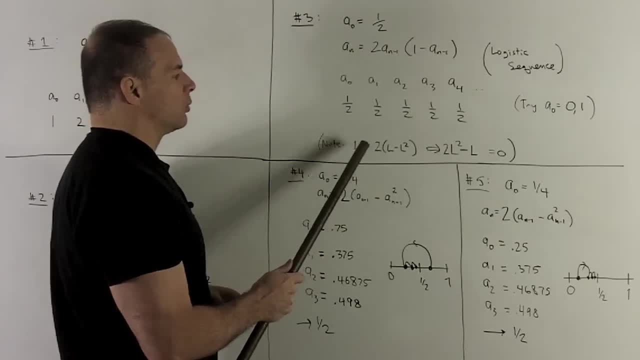 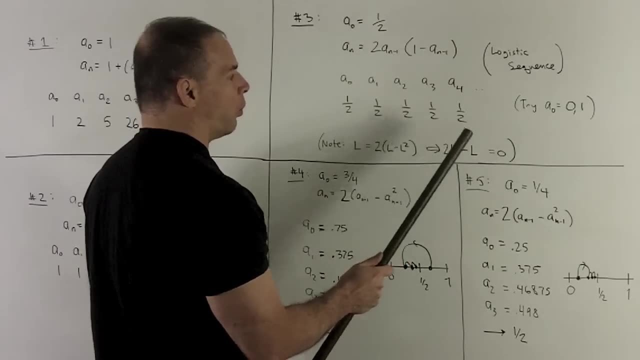 n or n minus 1 l. that's going to give me the equation: l equals 2 times l minus l squared, And then, if I solve for that, the zeros are going to be 0 and 1 half. Okay, magically, 1 half is doing something there. 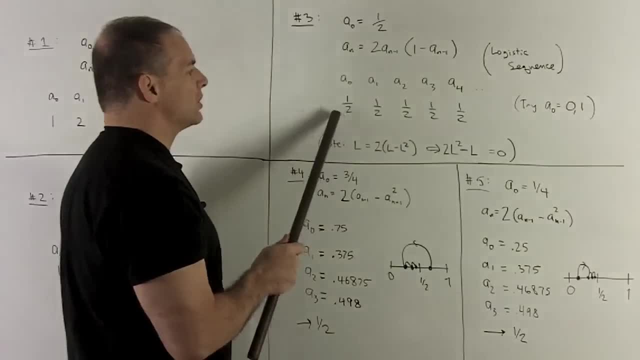 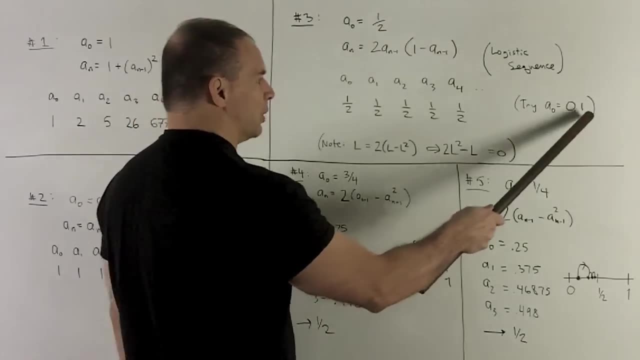 Okay, if you notice, if I put 0 in here, same thing. I start with 0, and then I just wind up producing a big string of zeros. All right, so I'll leave it to you to see what happens when you put a 1 in. 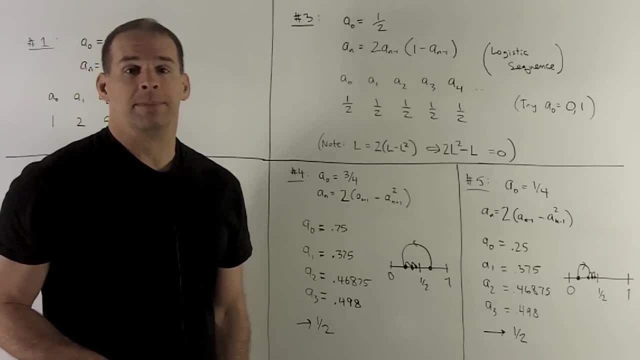 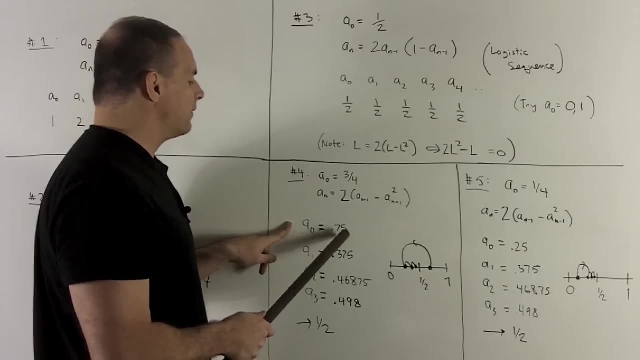 Now let's try some other points between 0 and 1.. So I'm going to go with 3 quarters. So we put 3 quarters in 0.75, and then you break out the calculator and just churn out a few terms. 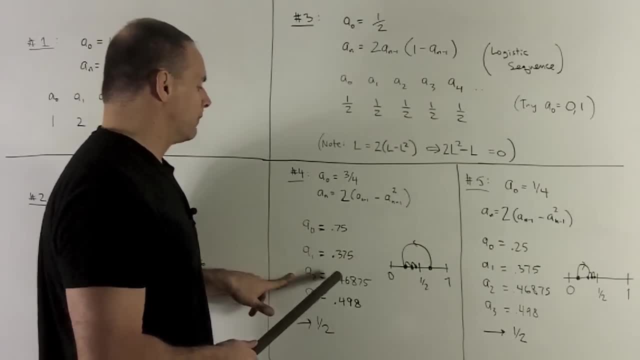 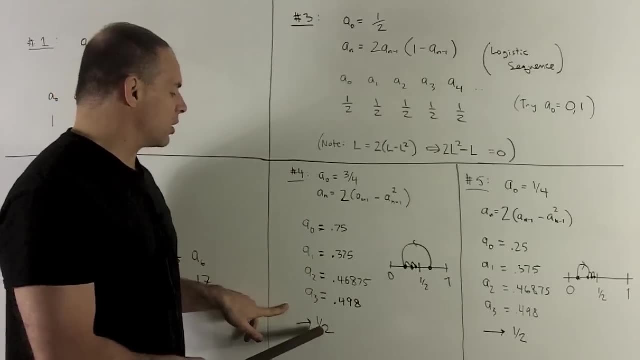 So the next term is going to be 0.375.. Next term is 0.46875.. Next term is 0.498.. And as you keep going and going and going, you're going to see that you're going to get closer and closer to a half, without ever actually getting there. 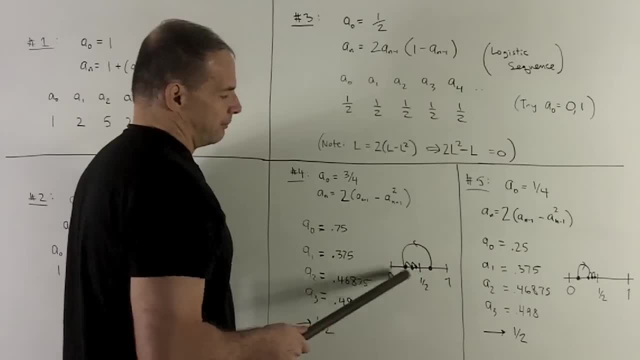 So the picture, If I put everything on, say, the x-axis, well, that's going to be starting at 0.75.. You're going to jump to 0.375, and then it just starts inching its way up to a half. 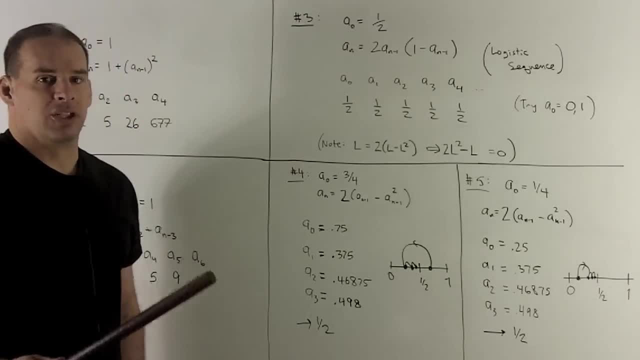 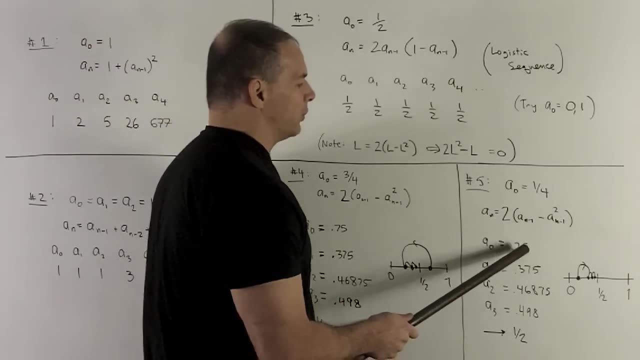 So that's the picture. All right, let's try another point. Let's go with, on the other side of a half 1 quarter, Same idea. I start with 0.25.. You put this in your calculator and start churning numbers.